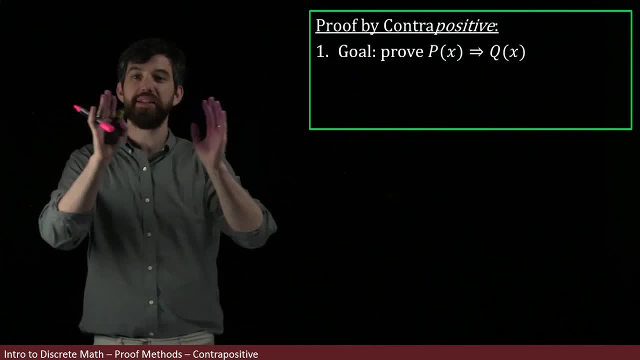 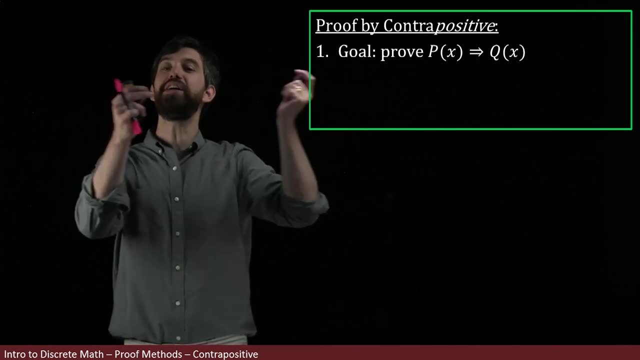 be to try to prove an implication. That's what I'm trying to do. I'm trying to show proven assumption leads to a conclusion, But what I'm going to do is treat this as the other way around. I'm going to know that P implies Q is the same thing as not. Q implies not P. That is I'm instead going. 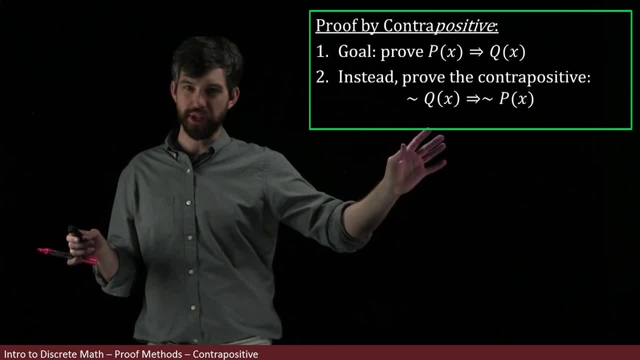 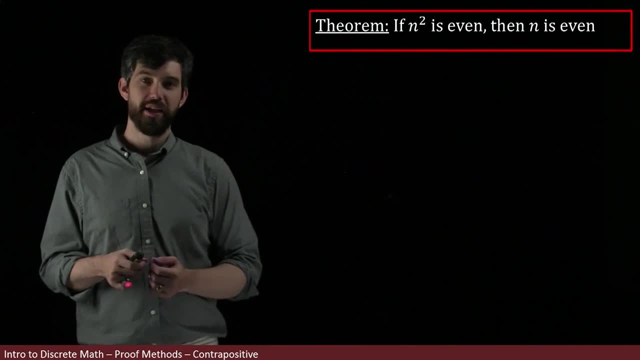 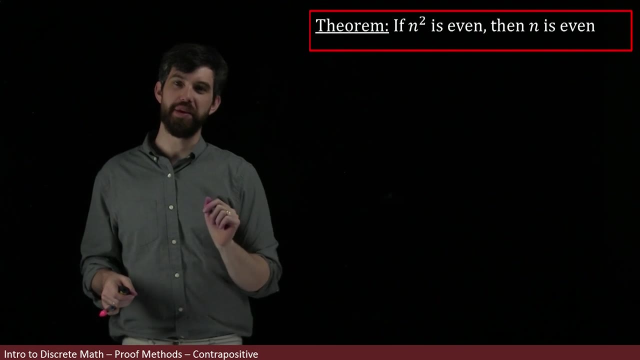 to go and try to prove the contrapositive. I'm going to try to prove not. Q implies not P, And that's the way I'm going to demonstrate that P implies Q. So let's see an example. In this theorem. I'm saying: if the square is even, then N itself is also going to be even, And I want to. 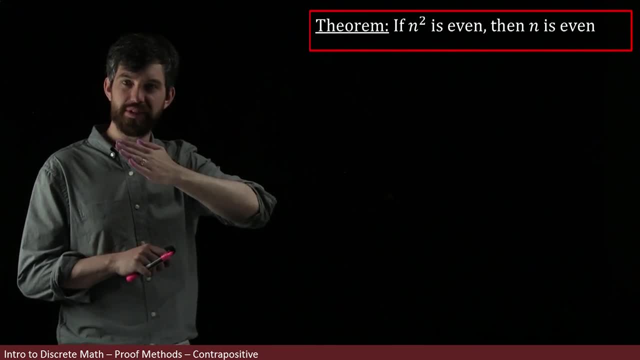 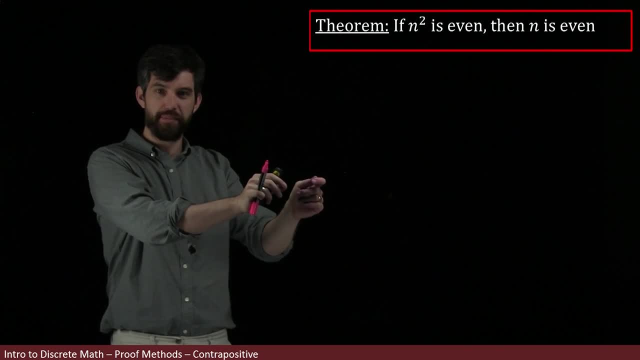 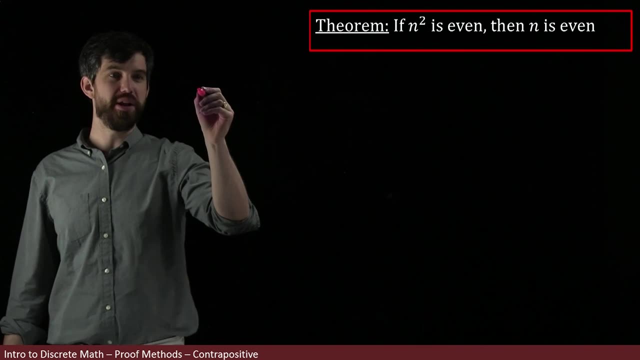 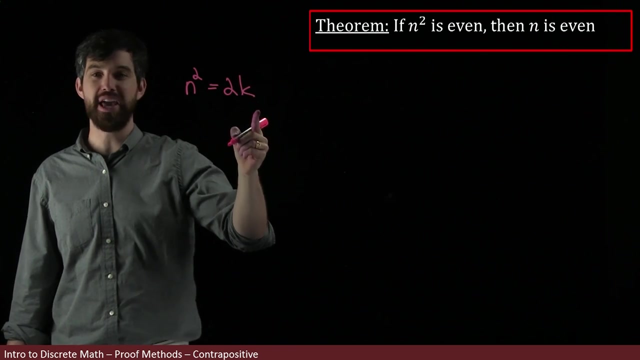 saying: if N squared is even, then N is going to be even. I'm going to just try to use a direct proof and show you why it might be challenging. So my assumption might be that N squared is even, which is going to be that N squared is going to be twice. some K for some K. I'm not going to write. 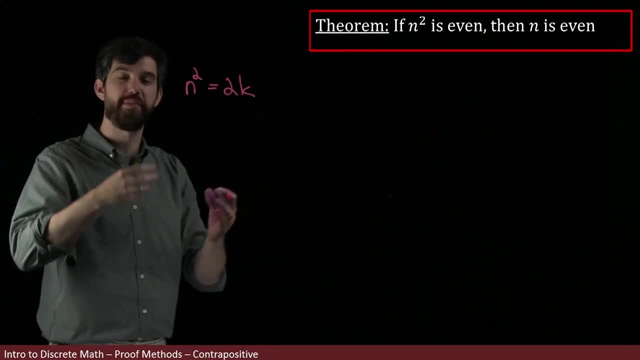 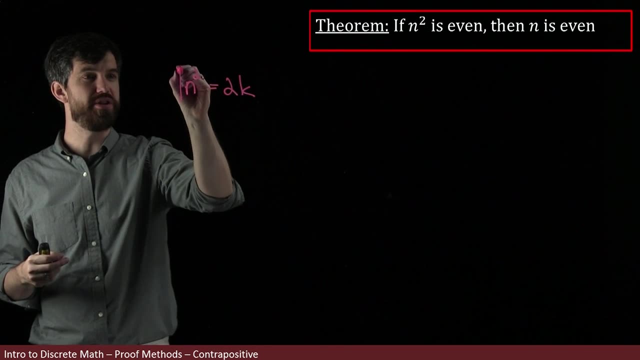 all my symbols down, because this is my playing around step. I don't have to be all that precise. All right, And I want to say that N? squared is even. And I'm not going to say that N? squared is even. I'm going to say something about N. I've got this square here, So maybe what I should be. 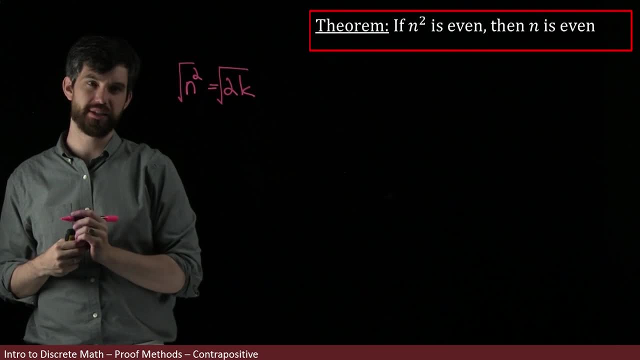 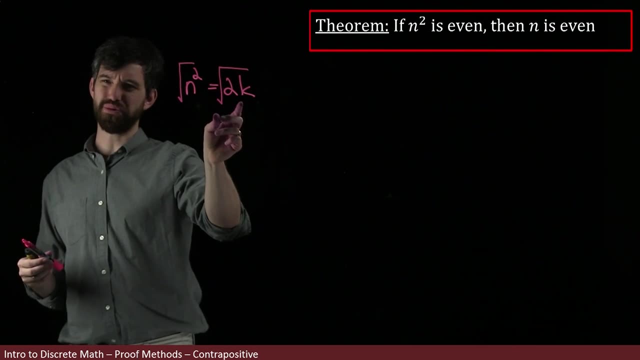 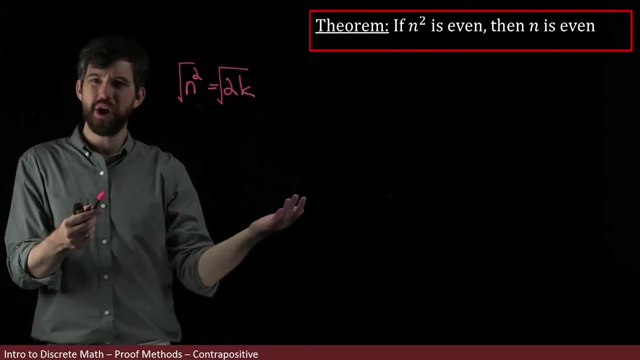 doing is taking a square root of both sides. That might give me my N if I took the positive square root, for instance, But then what I have is it being like equal to root two times root K, which doesn't really look anything at all like being. even. So, assuming that my N squared was even 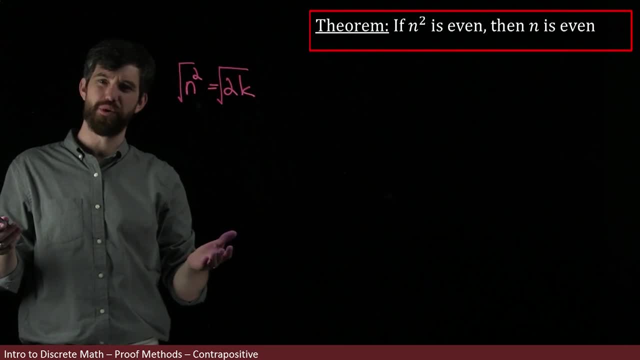 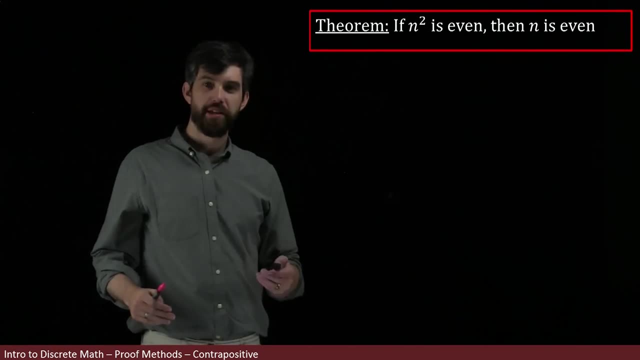 and taking square roots just didn't leave anywhere. It's got all this messy root two stuff floating around, So proving it directly seems a little bit challenging. So let's say let's get rid of that. Since proving this directly wasn't all that useful, let's try to. 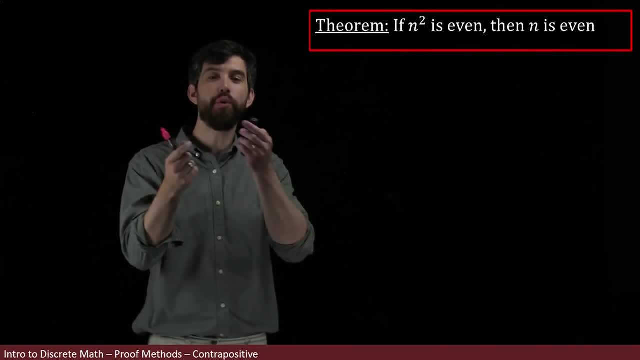 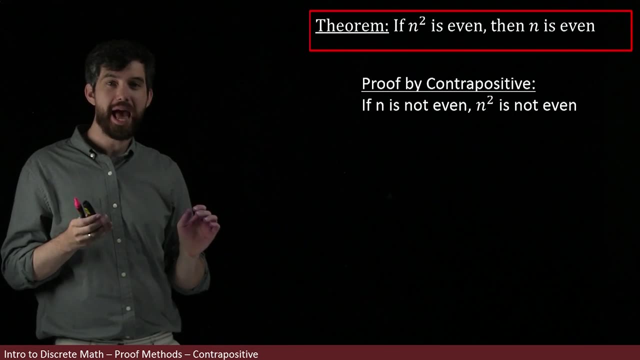 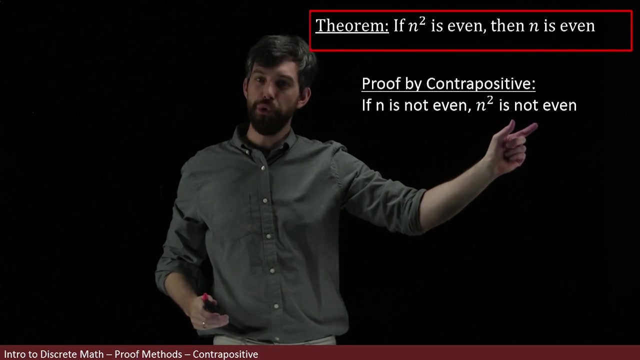 prove it by the contrapositive. We're going to do it the other way around with negations. So when I write it as proof by contradiction, by contrapositive rather, note what happens. First of all, the N squared is even and the N is even. they flip orders, but they also get two knots in.